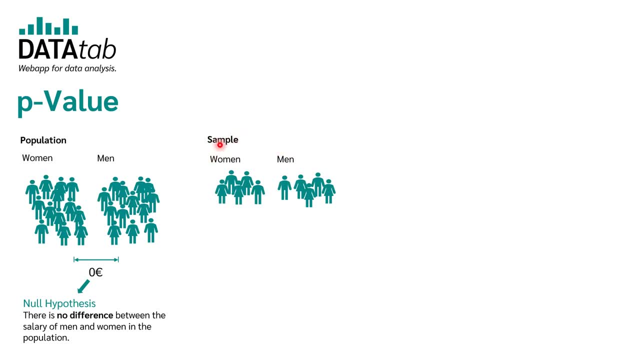 Therefore we need a sample. In this sample we also have the salary from women and men. So for sure, although in the population there is no difference between the salary In this sample, for sure there will be at least a small difference, It is quite unlikely. 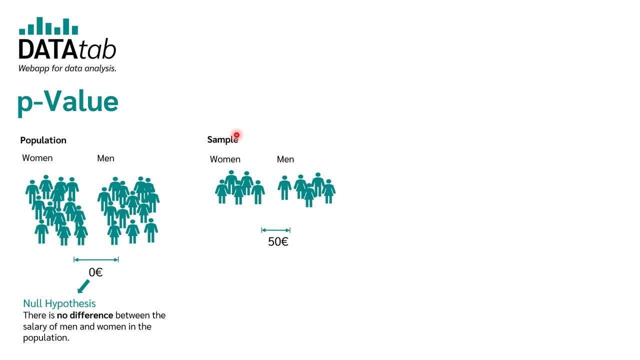 that the difference will be zero. For example, in this sample, the result could be that the difference is 50 euro or 150 euro, or 150 euro, 250 euro, even if there's no difference in the population. But again, the assumption is there's. 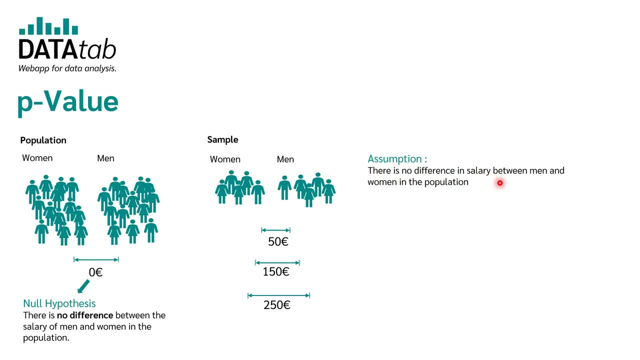 no difference in the salary between men and women in the population. And now we will come to the p value. The p value tells us how likely it is to draw a sample in which the salary of men and women differ by more than 50 euro. Or the p value tells us how likely it is to draw a sample in which the 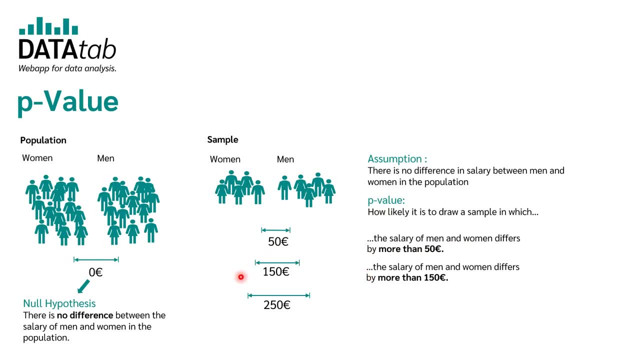 salary of men and women differ by more than 150 euro. Or the last example: the p value tells us how likely it is to draw a sample in which the salary of men and women differ by more than 250 euro. So again, we assume that there's no difference. 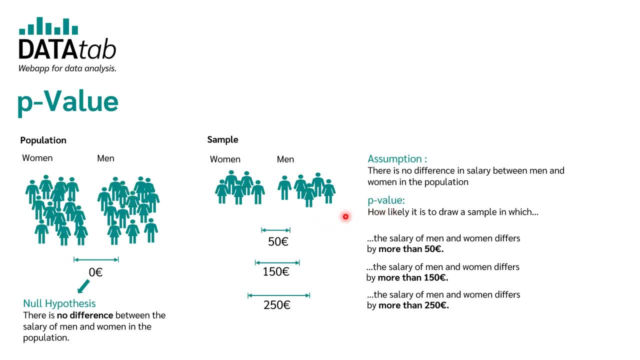 in the salary between men and women in the population. And now we will come to the p value. The p value now tells us how likely it is to draw a sample in which the difference between men and women in salary is 250 euro or greater, although there's no difference in the population. 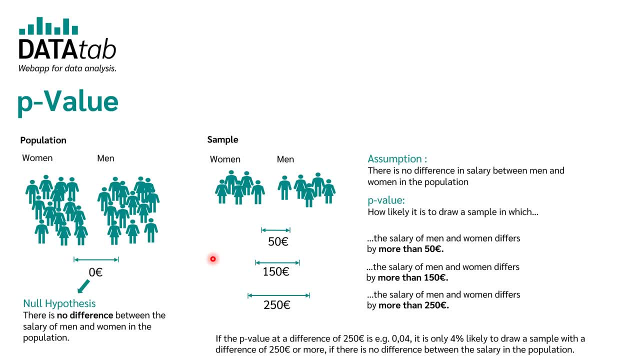 For example, if we are using data tab to calculate the p value and let's say, for the salary difference of 250 euro there's a p value of 0.05, and what does it mean If the p value at a difference of 250 euro is, for example, 0.05? 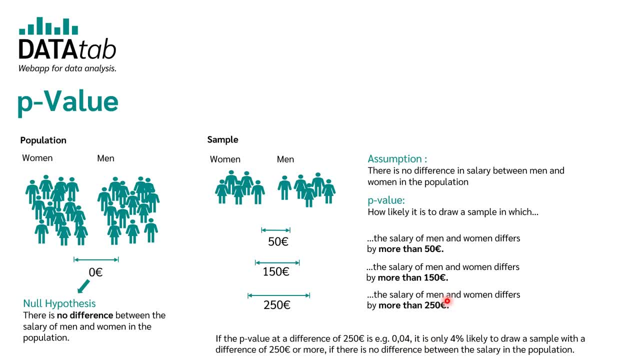 it means that only five- it is only five percent- likely to draw a sample with a difference of 250 euro or more if there's no difference between the salary in the population. So if there's no difference in the population, it is only four percent likely to draw a sample in which the difference in the salary is more than 250 euro. 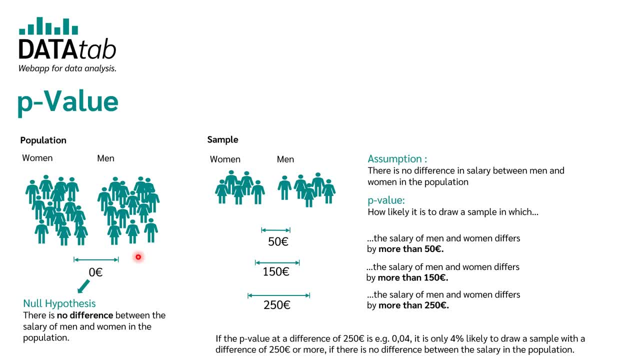 So if the p value is quite low, for sure we can ask if the null hypothesis is true in the population. Maybe the difference in the salary difference is not zero in the population. So and now we come to the question: at which point is it unlikely enough to reject the null hypothesis? 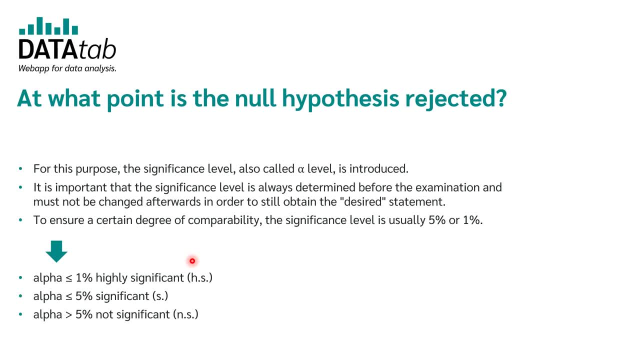 Therefore, we come to the question: at what point is the null hypothesis rejected? For this purpose, the significance level, also called alpha level, is introduced. It is very important that the significance level is always determined before the examination and must not be changed afterward in order to still obtain the desired statement, To ensure a certain degree of 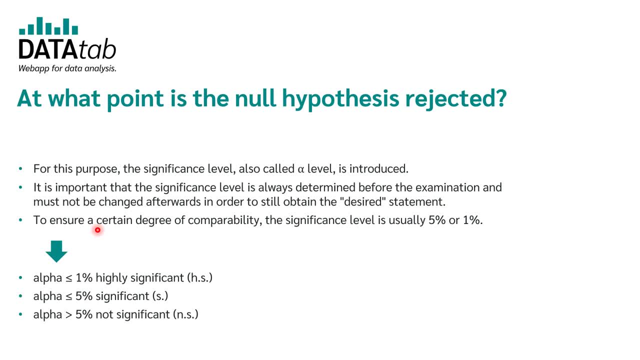 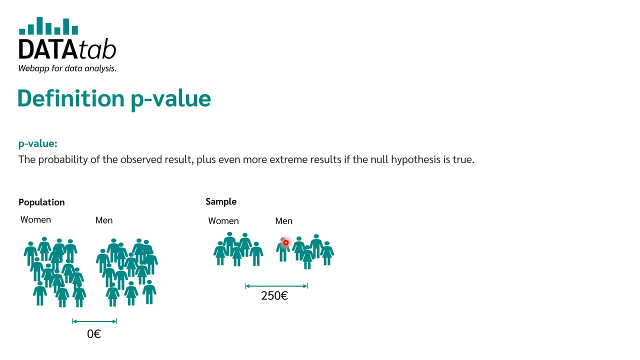 comparability. the significance level is usually five percent or one percent. The alpha level below one percent is highly significant, below five percent is significant, and above five percent it is not significant. So, and now we will come again to the p-value. The definition of the p-value is that the probability of the observed result. 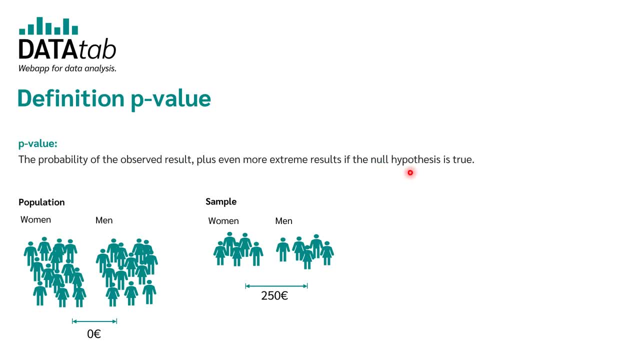 is less than or equal to zero. if the null hypothesis is true- And let's have a look at our example again- What does this mean? If the null hypothesis is true, is that we assume in the population there is no difference between the salary of women and men. So we asked: what is the probability that we draw a sample where the 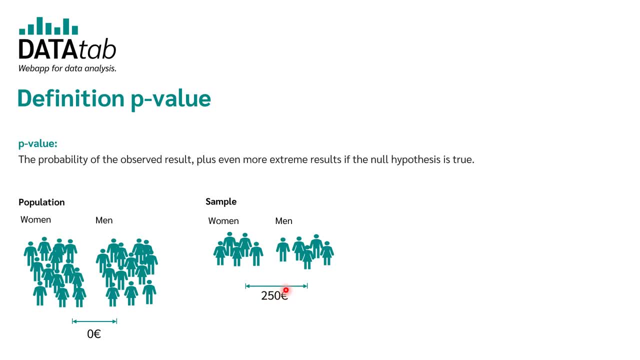 salary differ by more than 250 euro. If in the population there's no difference- For example, this could be four percent- Then this would mean it is only four percent likely that we draw a sample where the salary differ by more than 250 euro if there's no difference in the population.